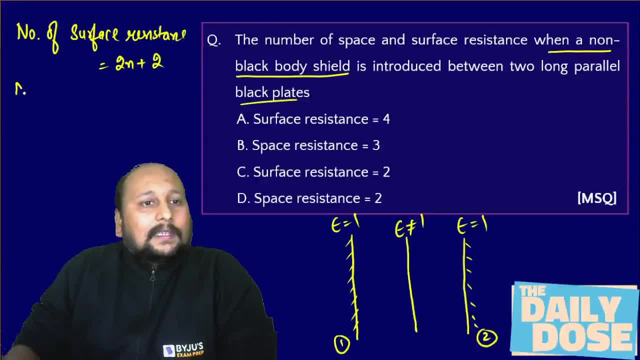 to 2n plus 2, right, and number of space resistance is equal to n plus 1.. This is the formulation that we are getting back of the mind, where n is definitely number of space resistance, Number of shields, Number of shield. In this problem, your n is equal to 1, because we are 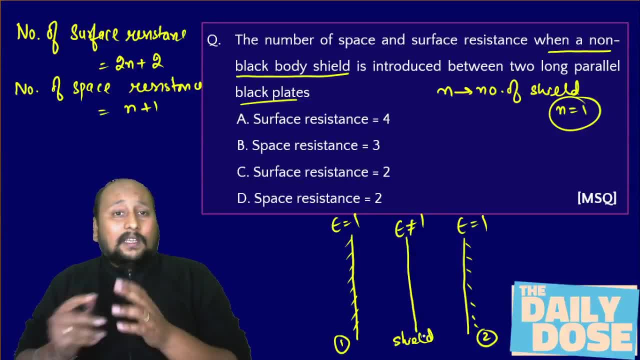 having one shield. This is your shield And I hope everyone knows. shield is basically introduced to reduce the rate of heat exchange between two surfaces. Now coming back to the question, if you try to apply n equal to 1, you'll be getting. surface resistance is equal to 4. 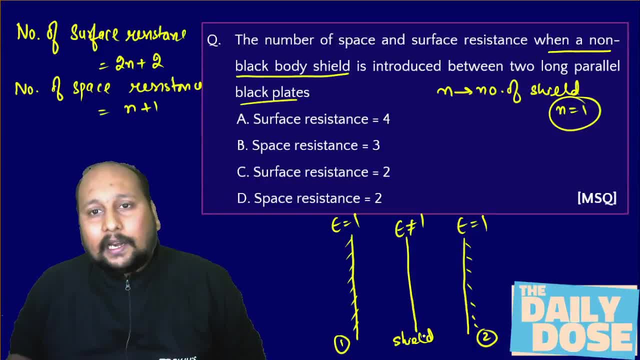 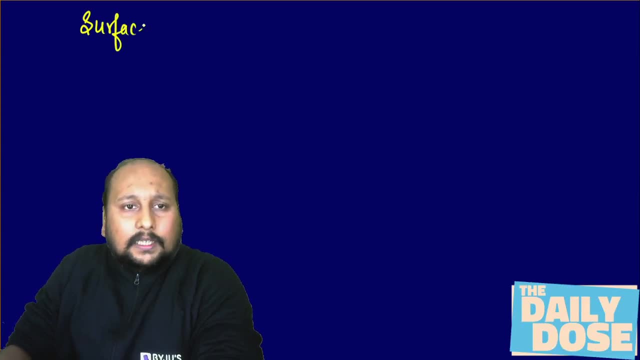 and space resistance is equal to 2,, which is incorrect, The reason being: you can only apply surface resistance to the black body. So let us understand what will be the answer for this. If I talk about the surface resistance Now, surface resistance basically depends upon the emissivity. 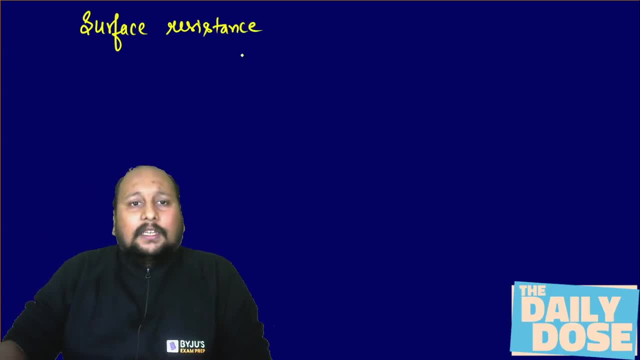 or the type of surface we are having. okay, because surface resistance is nothing but 1 minus emissivity upon emissivity into it. If I talk about the black body? If I talk about the black body, its emissivity is equal to 1.. That means its surface resistance. 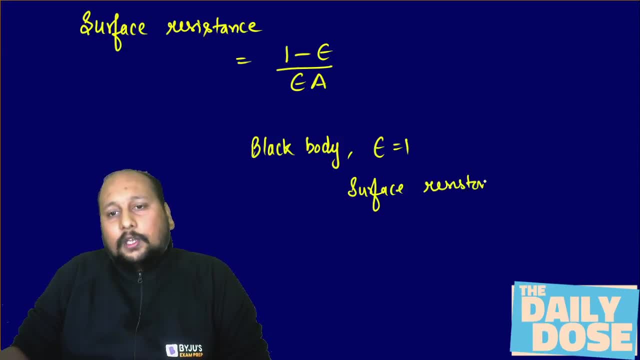 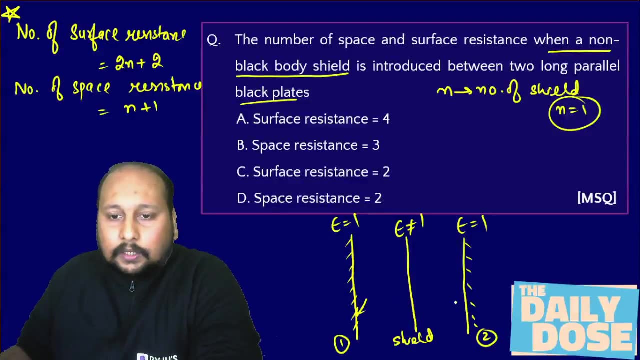 Surface resistance will be tending to 0, right. If surface resistance is equal to 0, that simply means you will be having a 0 surface resistance on both of the surface. 0 and 0, right. We will be only having surface resistance only on this shield, that is, surface resistance 1 and surface. 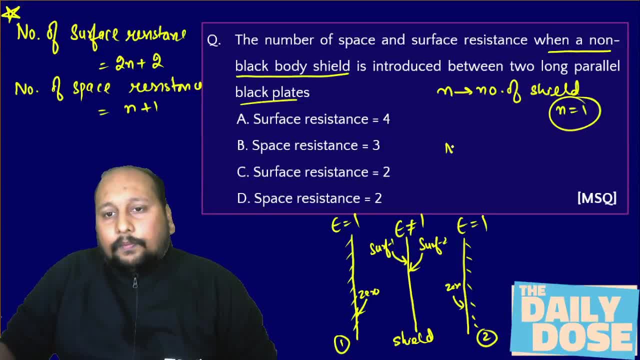 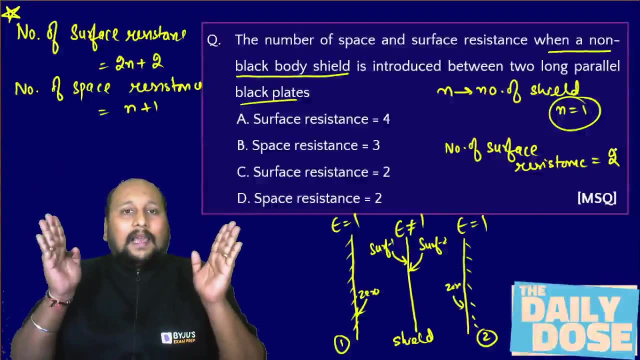 resistance 2.. So, in total, the number of surface resistance in this particular problem, in this particular arrangement, will be equal to 2, not 4.. Please make sure of this, because we are having two black surfaces and we know that black surfaces are always having 0 surface. 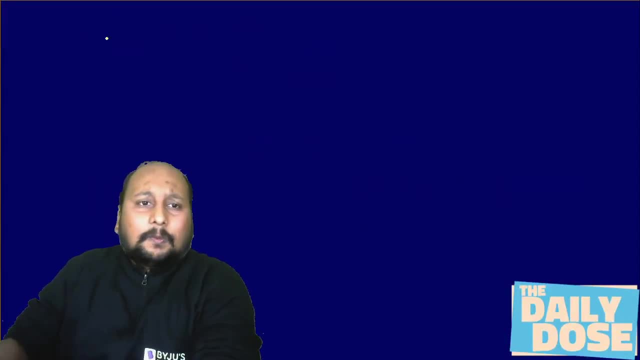 resistance. right, Talking about the space resistance. space resistance depends upon the space resistance depends upon very one important factor, that is, we call it as shape factor. okay, It depends upon the shape factor and definitely we know that shape factor is a shape factor. It depends upon how the surfaces are inclined to each other, or we can say what? 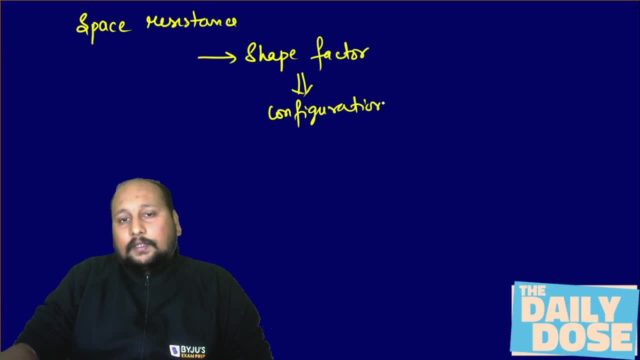 is the configuration of the surfaces right? That means, are the surfaces kept parallel or are they kept inclined? okay, Are we having a curved surface or are we having a straight surface? This is basically depends upon the configuration of the surface. So definitely. 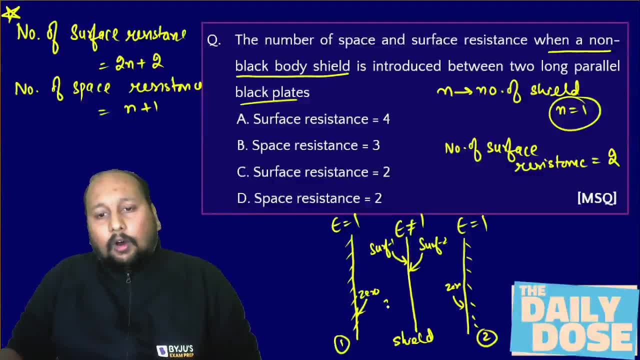 if it's a black body or non-black body, it is independent. You will always having a space resistance in between this. So number of space resistance is coming out to be Number of space resistance is coming out to be 2.. So in total, we are having two surface resistance. 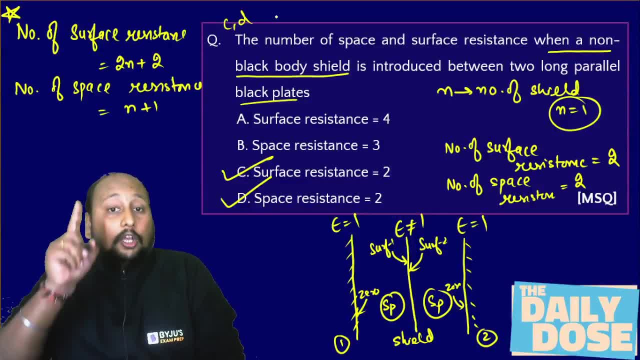 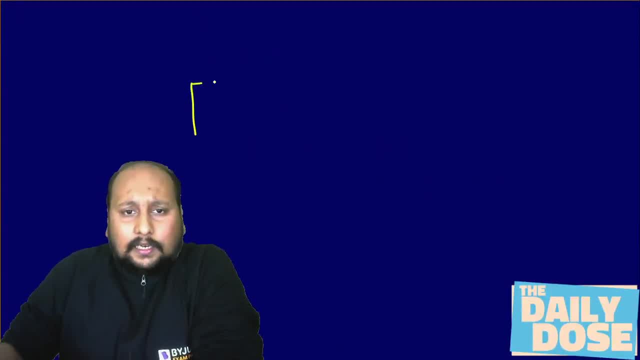 and two space resistance. Your final answer is C and D, not A and D, right, And we know very interestingly that if you are having two surfaces, let us suppose there are surface 1 and this is surface 2, right, And both surfaces are kept parallel. So both surfaces are kept. 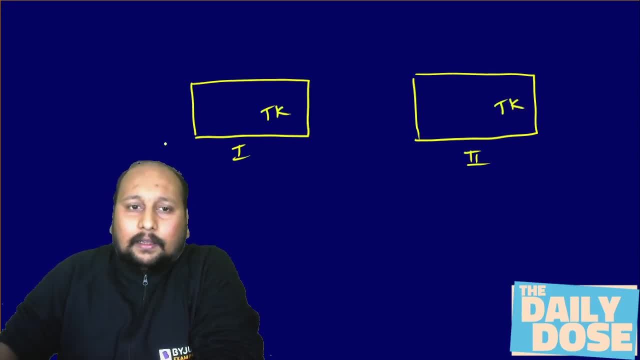 at same temperature- T kelvin. But this is a black body and this is a non-black body. So if we are having E1 emissions from here and E2 emissions from the second surface, both kept at same temperature, we can surely say that your emission from surface 1 will be. 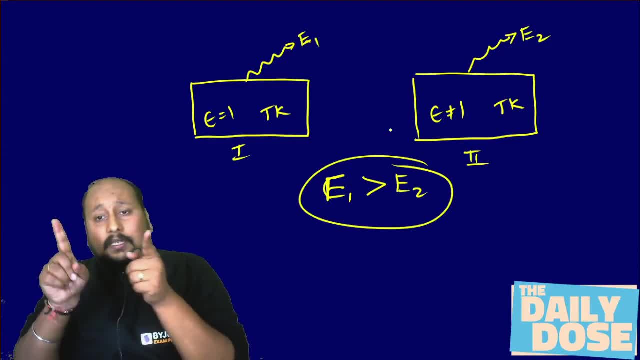 more than that of emission from surface 2.. The reason being because surface 2 is a non-black body, so it will be having a surface resistance which will be decreasing the amount of emissions from that surface. okay, So I hope so. now you have understood the concept of surface. 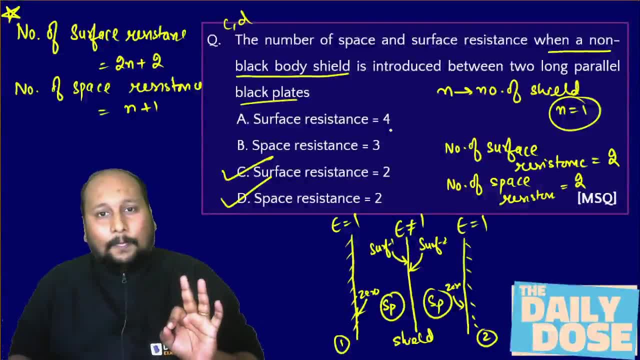 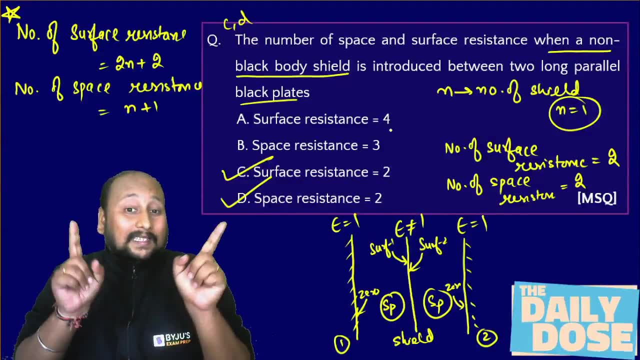 resistance, space resistance and the black body. So combine these three concepts, we are able to solve this question. So final answer is option C and option D, that is, surface and space resistance. okay, So this is all about today's daily dose from the radiation. 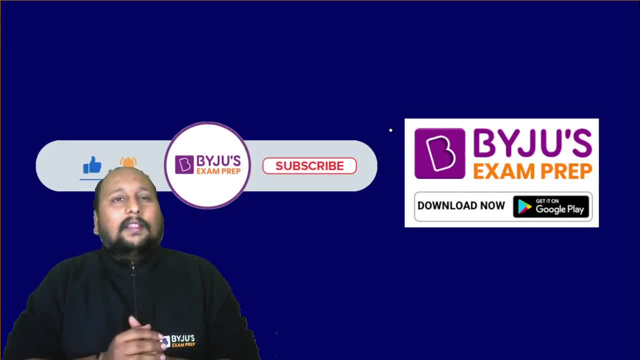 heat transfer. I hope you all enjoyed this, So please do like this session and please do subscribe to this channel for all such awesome content, for all our videos, Thank you. So this is Suraj Kopi signing off from your own bi-use exam prep. Thank you.